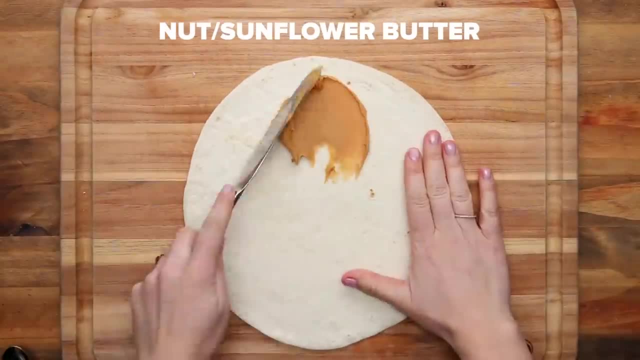 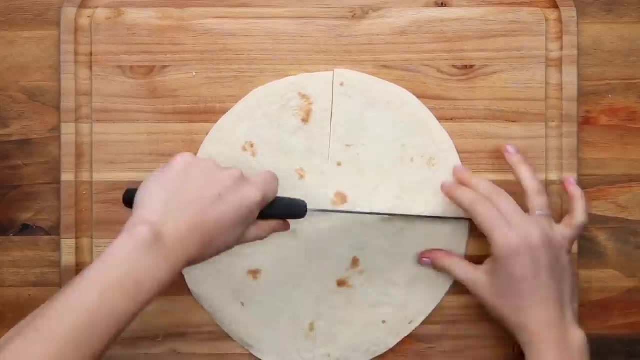 Did you like this? Did you like that? Like, can I put this in your lunch tomorrow too? And if I get an excited, yes, I know I've done a good job. By no means do you have to follow exactly what is in the video to a T. 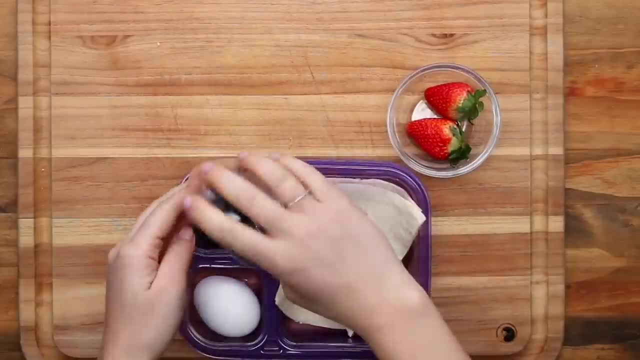 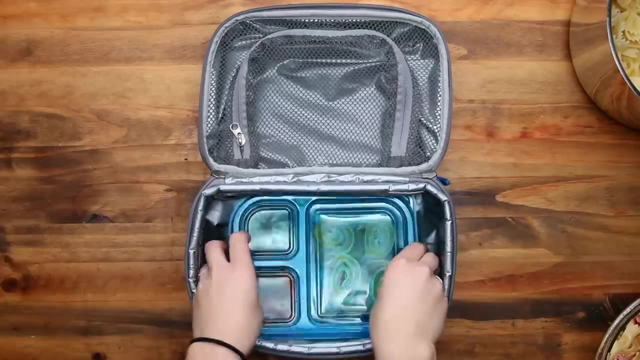 You can customize it to make whatever you think your child would like. Obviously, not every kid is going to like hard-boiled eggs in their lunch, but that's okay. You can put in something else that you do know that they like. That way, you can provide them with a lunch that you know they're going to enjoy. 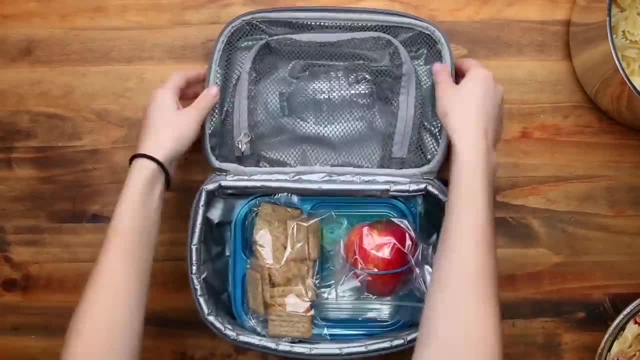 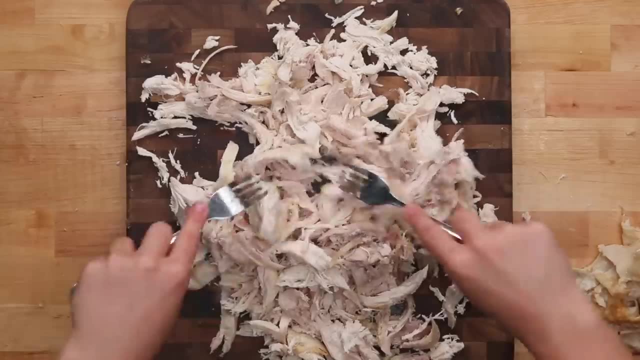 but is also going to give them sustainable energy throughout the rest of the day. Another way you can meal prep is by using leftover chicken, or you can buy one chicken, shred it up and make your lunches from there. Chicken is one of the most popular meats in the world. 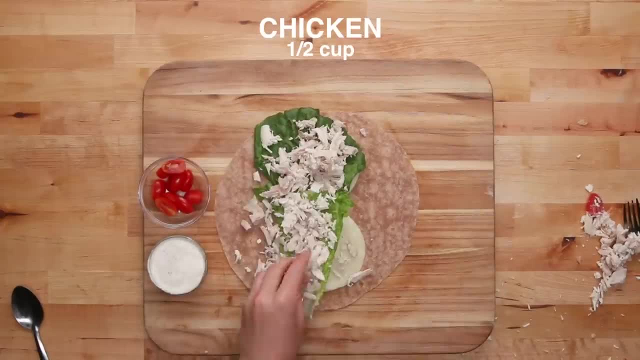 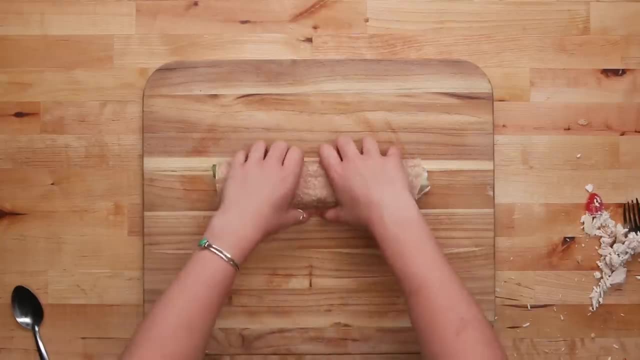 and just about every kid I know will eat chicken. There's a variety of recipes that you can make with chicken, which is why it's perfect for meal prepping for kids' lunches. Like I said before, you can use these as jumping-off points. 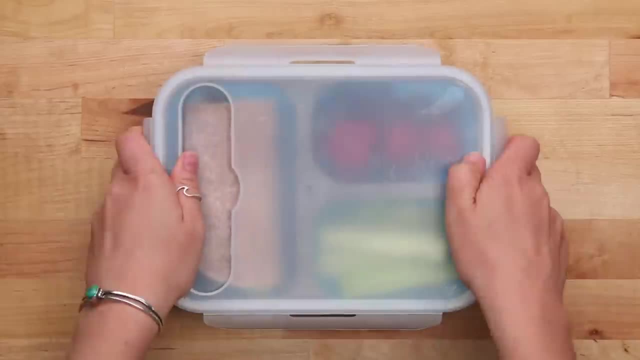 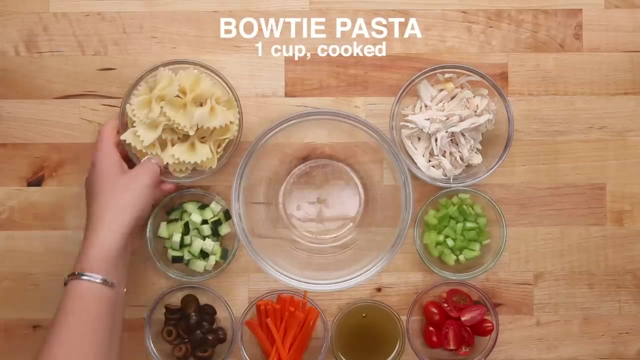 If your kid doesn't like chicken salad, you can make your own version or mix it up with your favorite family recipe. This is just another way to optimize your efficiency. in the mornings, You just have one solid protein and you expand on it from there. 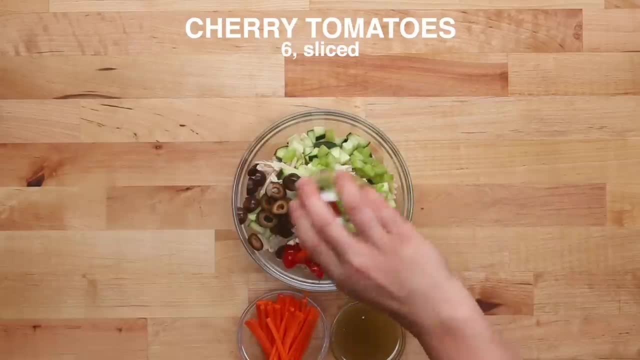 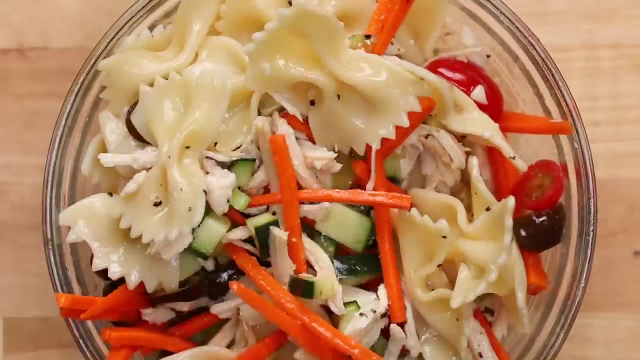 and you can really go anywhere with it. Just make sure to remove all the bones and cartilage and shred the chicken. really well, Growing up in my house I hated eating leftovers, so my mom would get sneaky and she would turn the leftovers into something new. 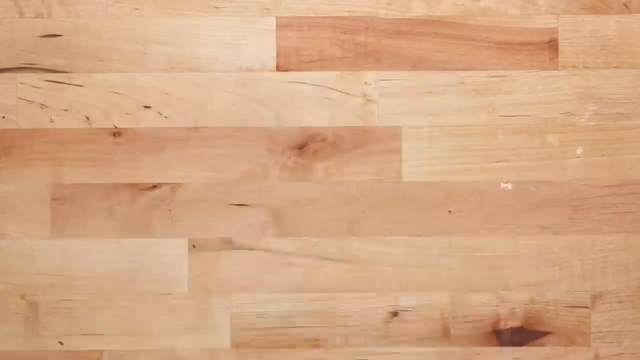 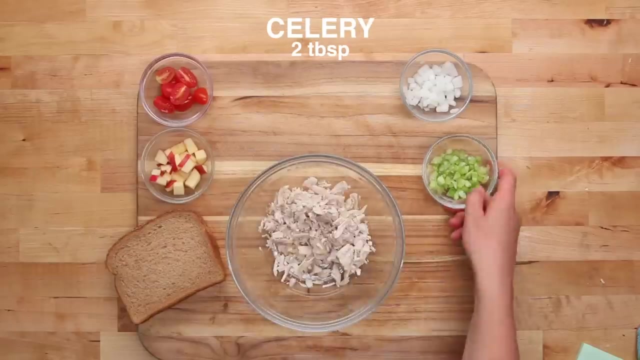 so I wouldn't even know that I was eating leftovers for lunch, So that was something that really inspired me to make this video and to pay homage to my childhood, as well as my upbringing. If it wasn't leftovers, my lunches were typically pretty boring and the same every day. 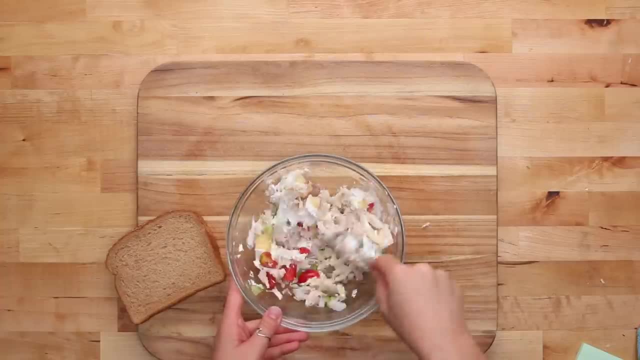 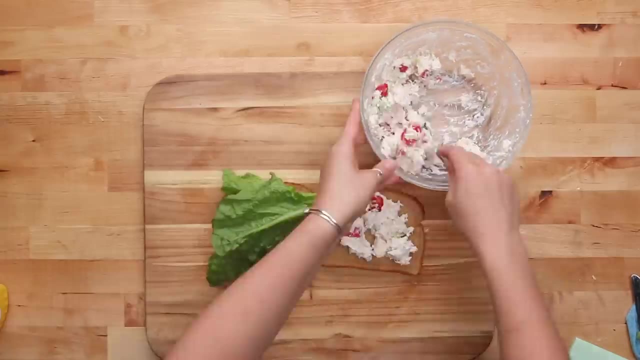 so I didn't want the same for my niece and nephew, and that's why I put in a lot of effort to make their food exciting and fun to eat. My niece is only six, so having a full day at school is a really long time for her to go without having a snack every five minutes. 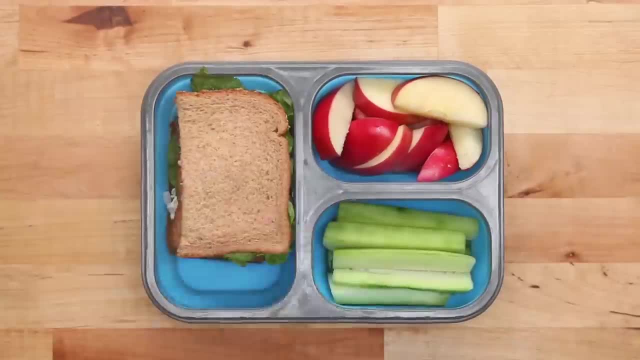 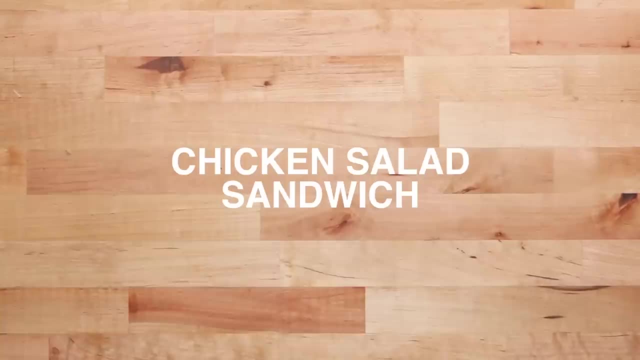 I really like making sure that she has healthy choices for her lunch every day. Making a lunch that she brings home with the box totally empty is such a satisfying thing When you're that age. lunch is such an exciting time of the day, and it's even an exciting time of the day for me as a 25-year-old woman. 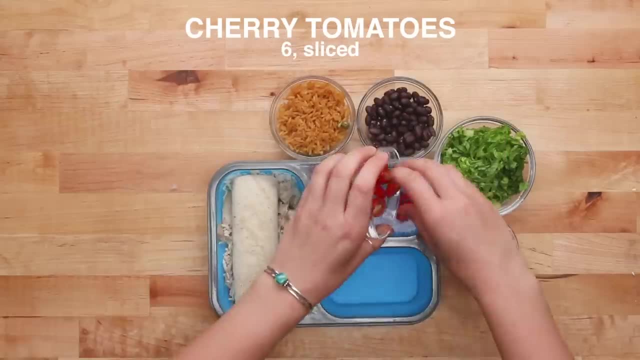 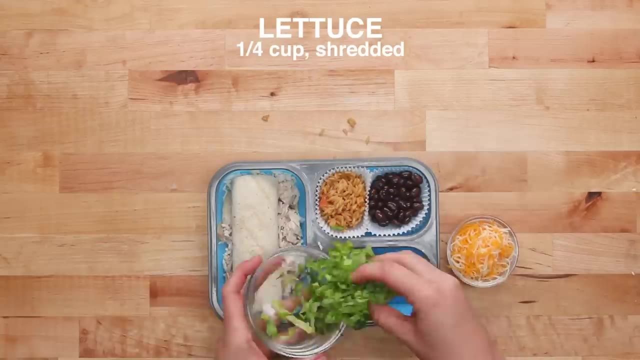 One of my favorite things to do that my mom used to do for me is to leave notes in their lunches with funny little sayings, and I absolutely think that I'm the funniest aunt in the whole entire world because I leave the cheesiest corniest notes. 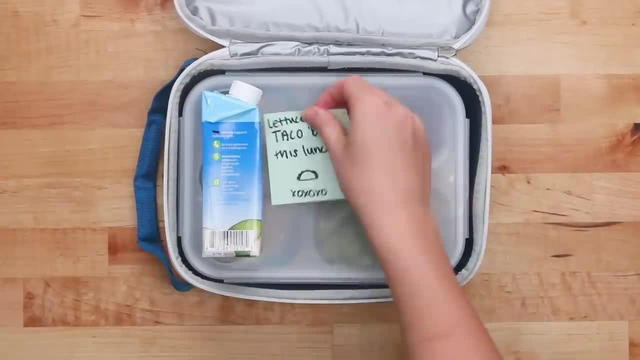 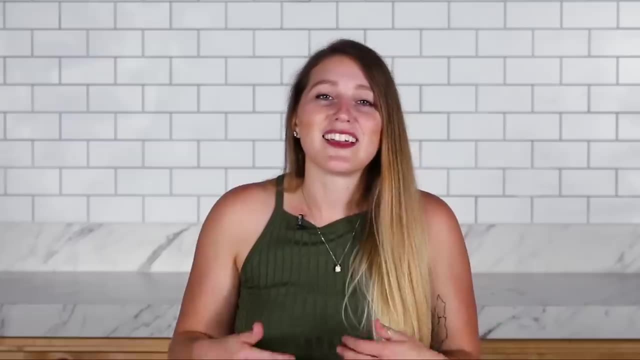 and I crack myself up as I'm writing them every morning. I like to add puns on little notes in their lunches and I think I'm funny, but I don't know if anyone else does. But like, come on, I believe in you. 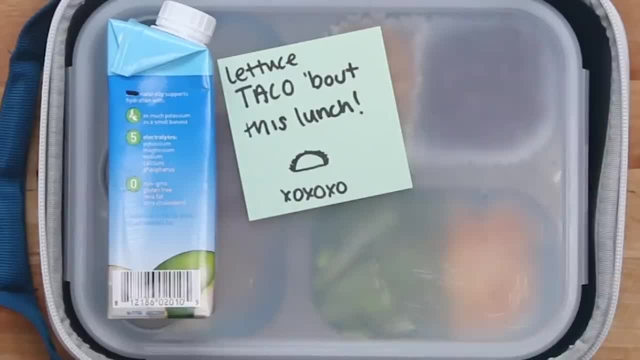 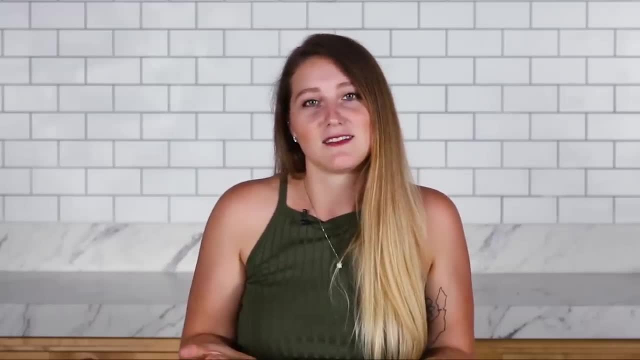 Come on Like: let us taco about it. You've been a good kid today. I'm funny, Give me the credit. I'm funny For my nephew, since he's only three, he can't really read, but my niece is starting to be able to read. 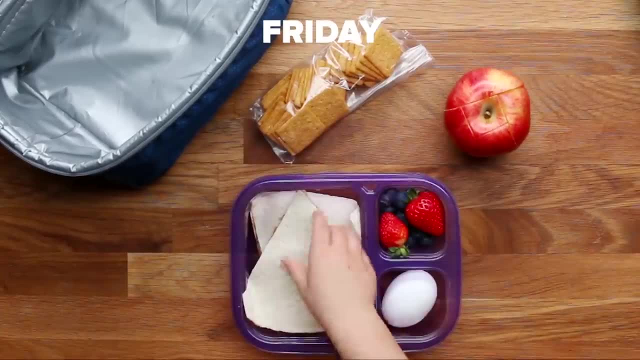 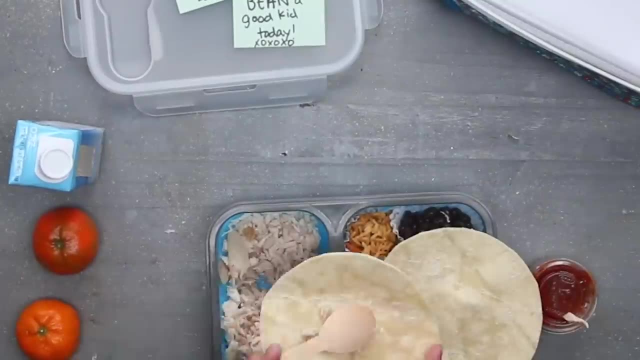 and she either gets my jokes or kind of looks at me in disappointment like, oh Auntie, that was a bad one. I always thought it was so special when my mom would put notes in my lunch, because it was just a little reminder from her to me. 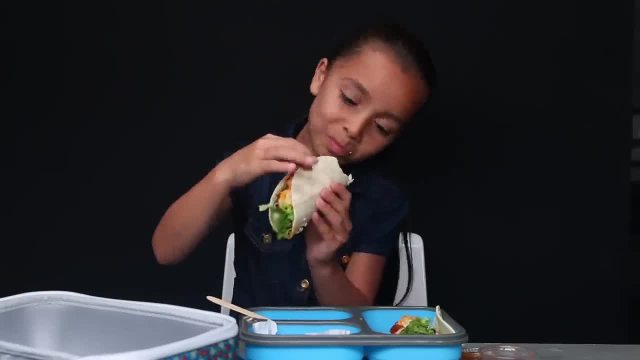 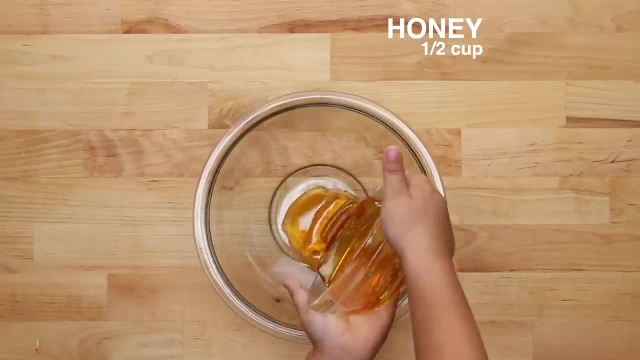 that she loves me and cares about me. So I'm carrying on that tradition with my niece and nephew. These cereal bars are the best snack for any time. You can grab them and go for the morning. You can put them in a lunch. 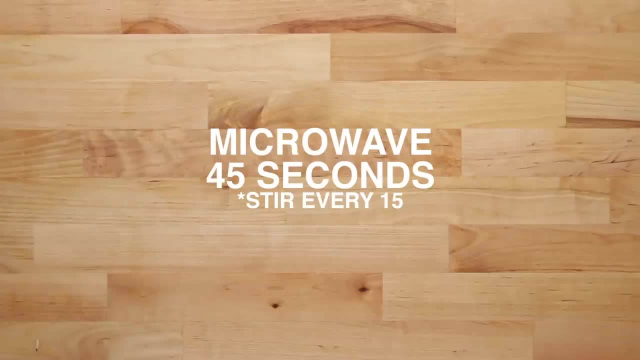 You can have them as an after-school snack. They really are the perfect food for any time of day. When you're making these, it's a perfect opportunity to involve your child in the cooking process with you. It's the best when you see how proud they are of themselves. 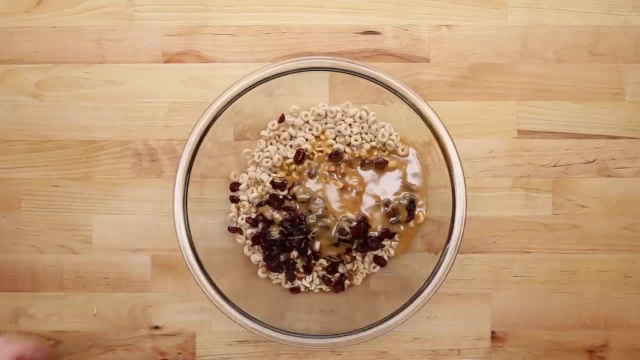 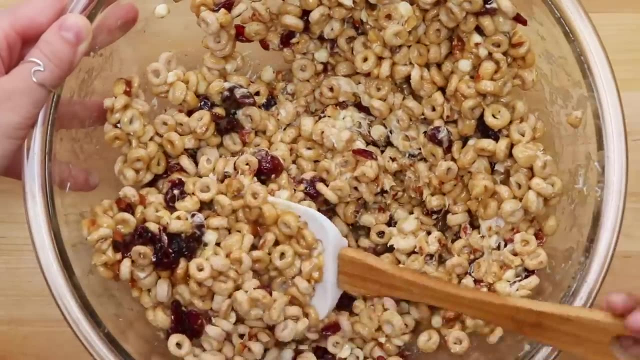 And you see a big smile across their face. My coworker, Hannah's son, Jackson, helped me make this and he's usually my sous chef in Tasty Junior videos. This particular day, he was really upset that we were putting the yogurt chips in the mix. 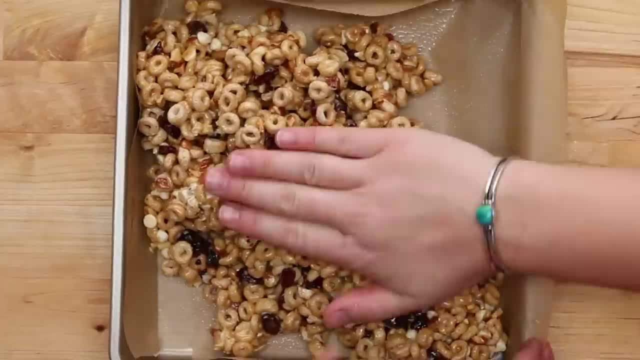 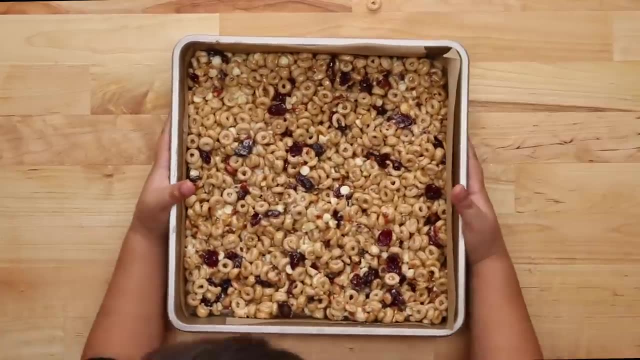 I had to tell him they're part of the recipe and we have to put them in. but you know what we can do. We can make a batch separately, just for you that doesn't have yogurt chips in it, And he really enjoyed having his own little version. 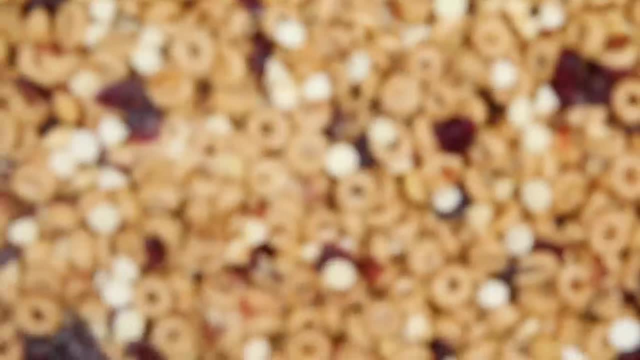 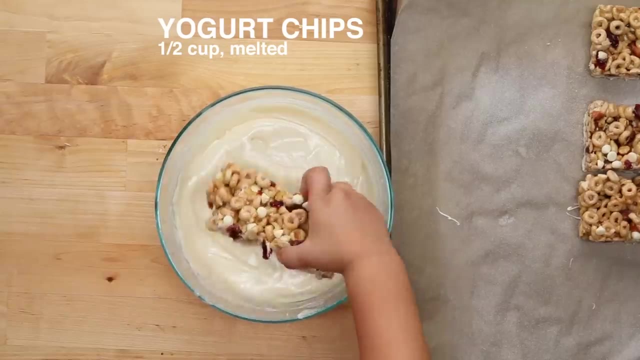 At the time I was a little frustrated with him because he was changing my vision, but he really taught me a lesson. He taught me a valuable lesson in that you should always customize your recipes to your own preference. Another reason these are great is because you can wrap them up. 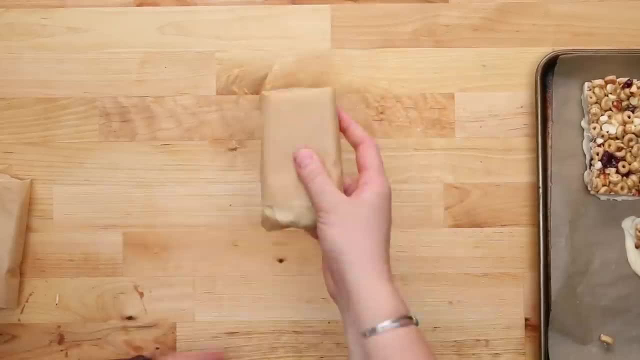 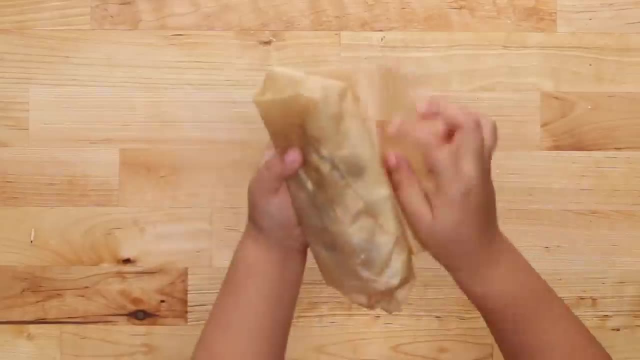 and save them in your fridge for about three months before you'll need to toss them. These are just another way for you to save time and also this way you know what ingredients are going in, compared to the mystery ingredient sugar-filled bars that there are out there today. 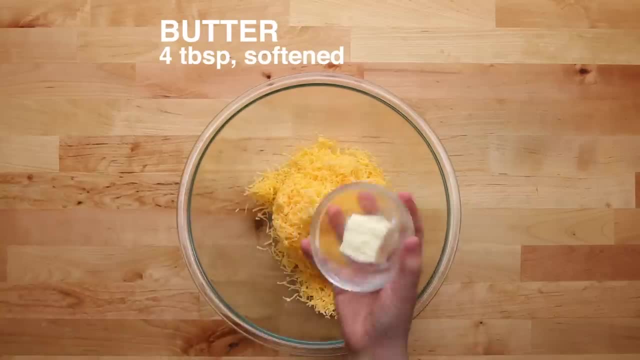 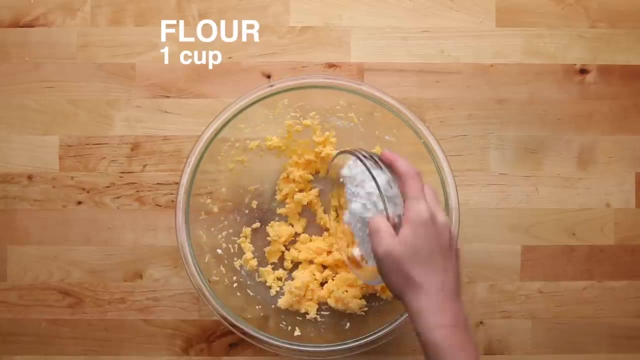 Now with this snack. I can't tell you exactly what they're based on, but it starts with cheese and it's a great snack, But we'll just call them baked cheese crackers for now. My favorite part about this recipe is that. 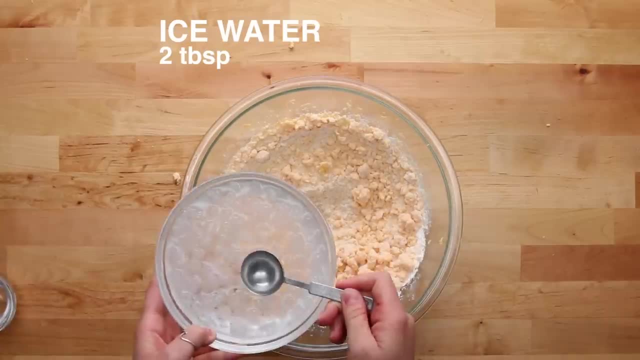 it's four ingredients. It really doesn't take that long to make Just a little bit of effort, but the effort is worth it. These are something that I make for myself all the time and they pair really well with Chardonnay, by the way. 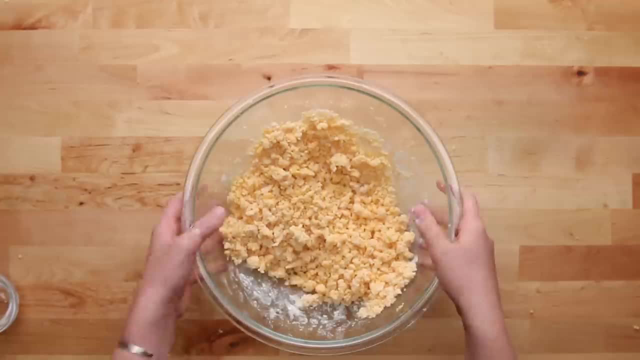 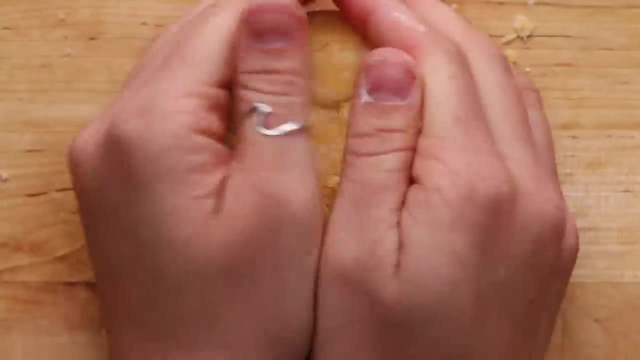 They're lighter and they have a really satisfying crunch to them. Have the kids help you cut out the shapes and put them on a baking sheet and poke a hole in the middle. When you use the cookie cutters, it just makes it so much more fun. 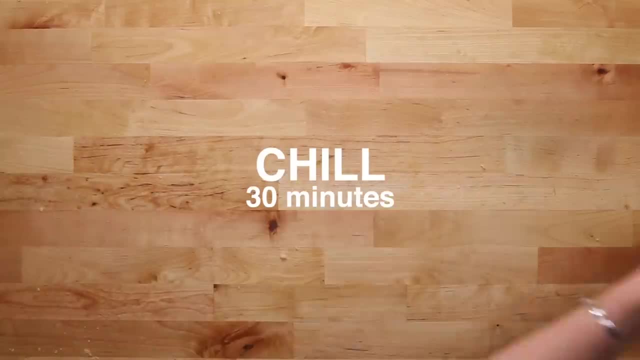 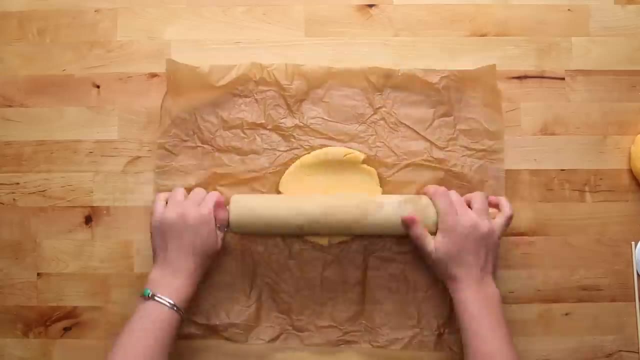 and so much more kid-like. You can add these into lunches, You can keep them for an at-home snack. You can hide them in the back of the pantry for yourself. Whatever you do, just make them. You can even play with the type of cheese that you put in them. You can do mozzarella Colby Jack American- No, don't do American Mozzarella Colby Jack, Pepper Jack if you're a little fancy. Or you can even amp up the flavor with a really great sharp cheddar. 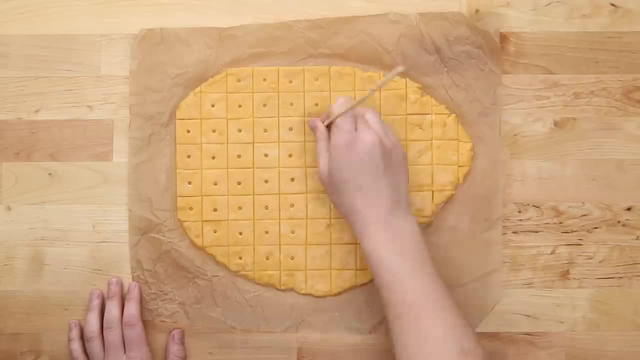 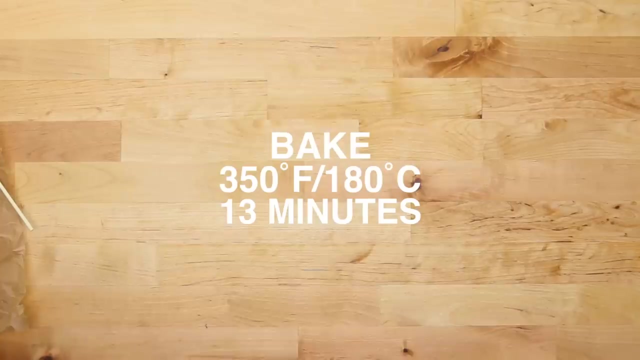 and you'll have really flavorful and delicious cracker. You can also use a cookie cutter and just keep rolling out the dough until you don't have any dough left, Just like last time. I told you guys that I do read the comments and, believe me, I know you can buy these in a box. 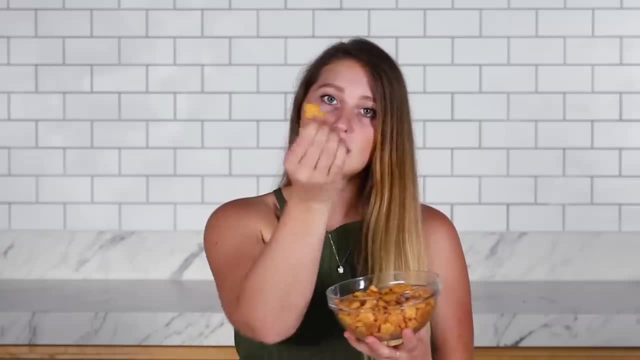 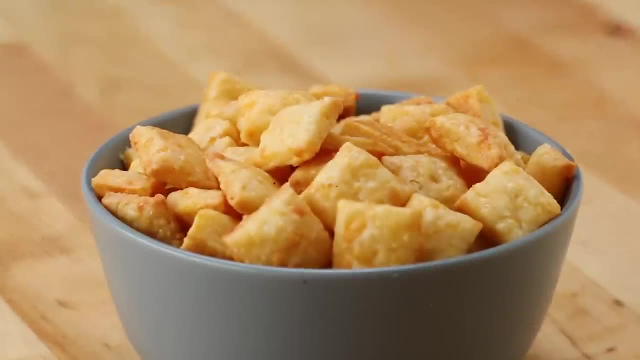 but making them is so much better and you can make the cutest little shapes and they taste ten times better. Promise, Go, make them. I mean, it's only four ingredients You probably have in your house right now. It's another surefire way of making sure you know. 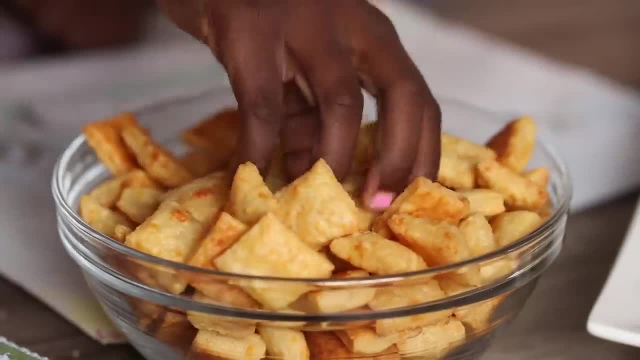 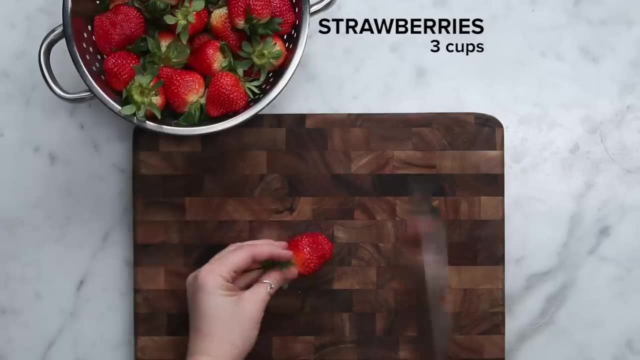 what your kids are eating and what's going into those foods. This is another four-ingredient, really easy snack. You could even really do it with three ingredients. You're really just dehydrating the fruit and that's what's taking so long. 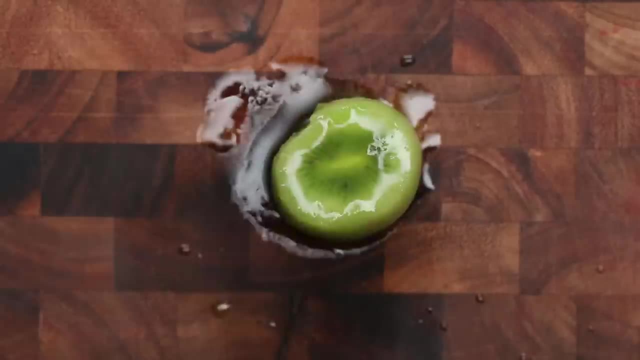 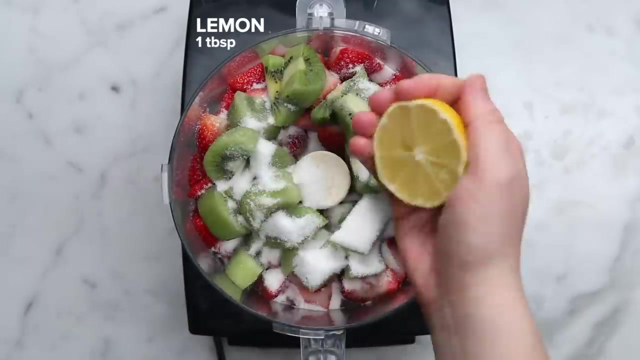 but the end result is worth it. If you were to compare these to rolls that you would buy at the store, you can look and see that there's far less processed ingredients. These are something that you can do in big batches. You can do two or three sheet pans at a time.